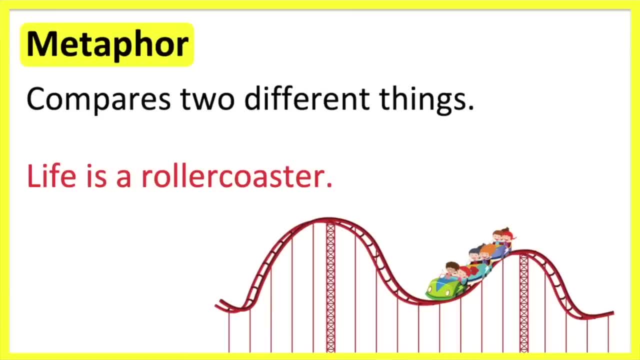 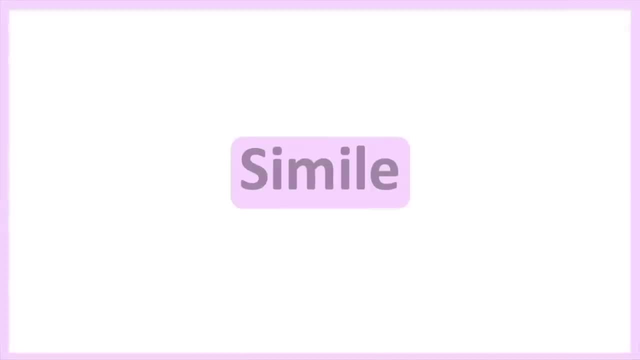 Remember that a metaphor is a figure of speech. This means that it shouldn't be taken literally, as the words in the sentence convey a different meaning. A simile compares two different things. We say that something is like or as something else. For example, Jim is as tall as a giraffe. 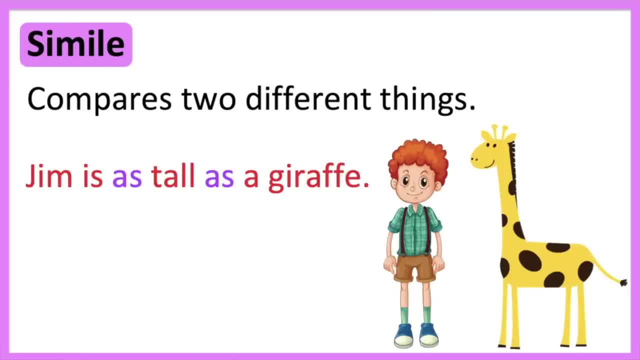 In this example, the simile compares two different things that are compared due to their common characteristic, which is their height, their height. So essentially I'm saying that Jim is very tall. The simile makes the sentence more interesting and creates an image in the reader's mind, rather than simply just saying Jim is tall. 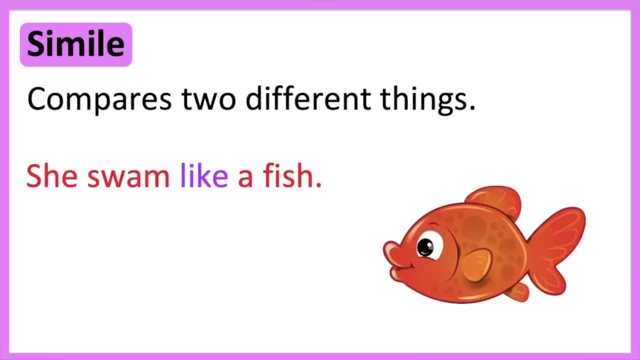 Another example is she swam like a fish. Again, this simile compares two different things due to their common characteristic, which is that they can both swim very well. Remember that a simile is a figure of speech. This means that it shouldn't be taken literally as the words in the sentence. 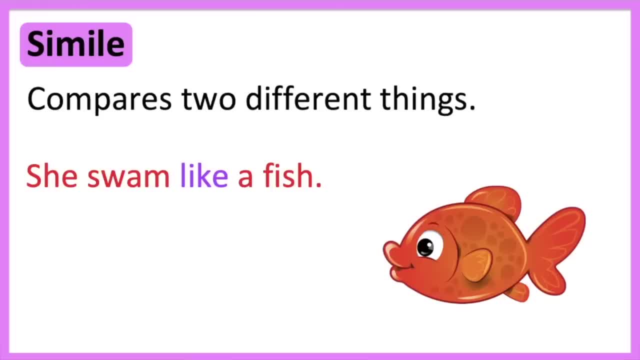 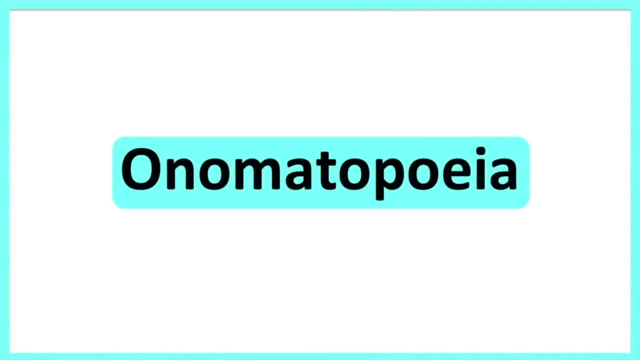 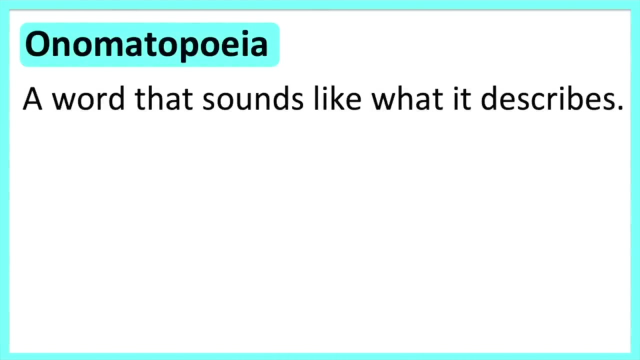 convey a different meaning. Lastly, remember that similes always includes the words like or as, So onomatopoeia. Onomatopoeia is a word that sounds like what it describes. It's a language technique used to make writing more interesting and helps the reader to hear the sounds in their minds. 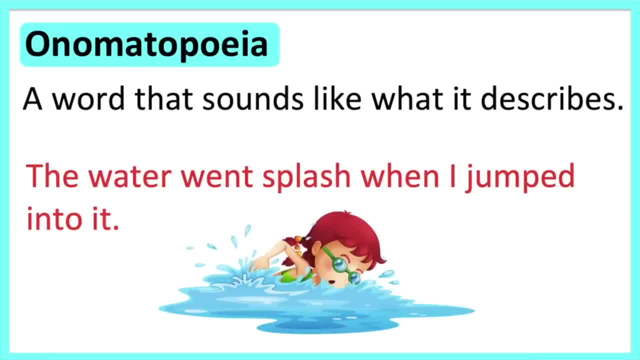 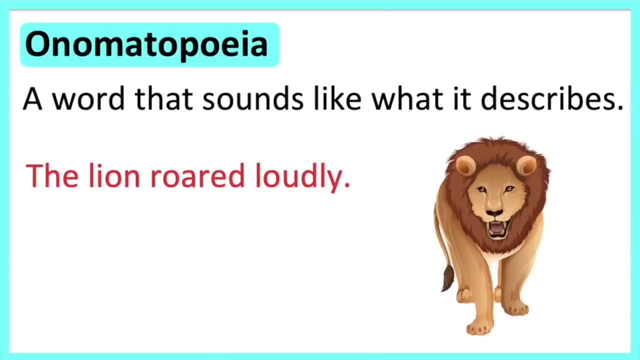 For example, the water went splash when I jumped into it. The emphasis is on the sound the water makes Splash. This is the onomatopoeia. The lion roared loudly. The onomatopoeia is roared. This emphasizes the sound the lion makes. Another example is the balloon popped. 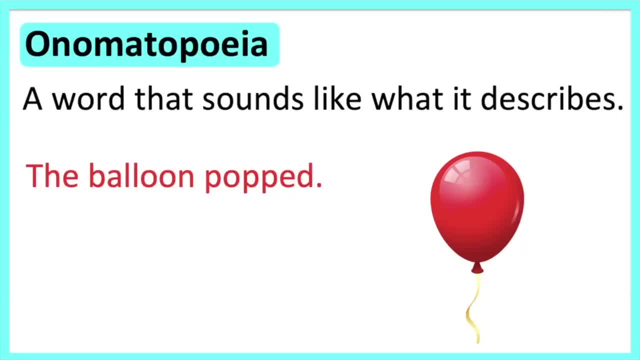 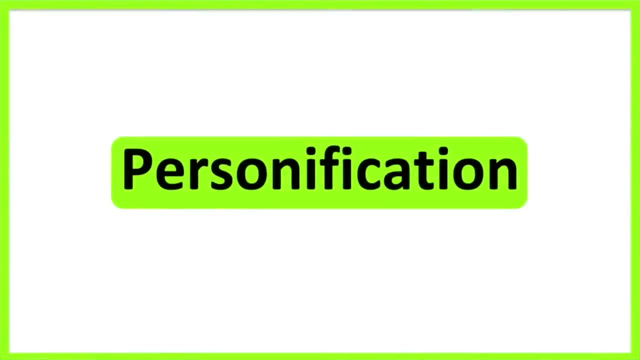 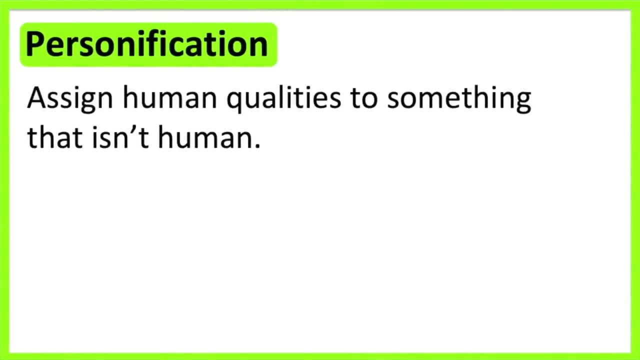 The onomatopoeia in this sentence emphasizes the sound the balloon makes Personification. Personification is when we assign human qualities to something that isn't human. These can be movements, emotions or senses. For example, the tree is dancing in the wind. 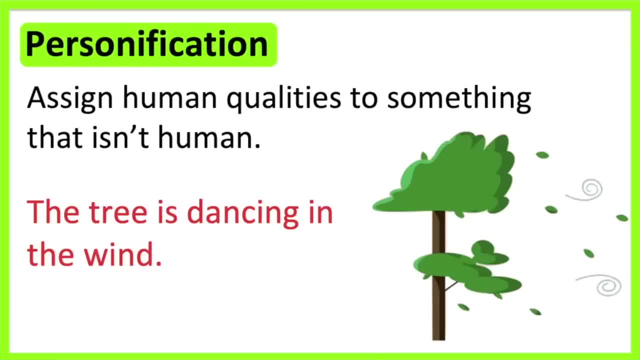 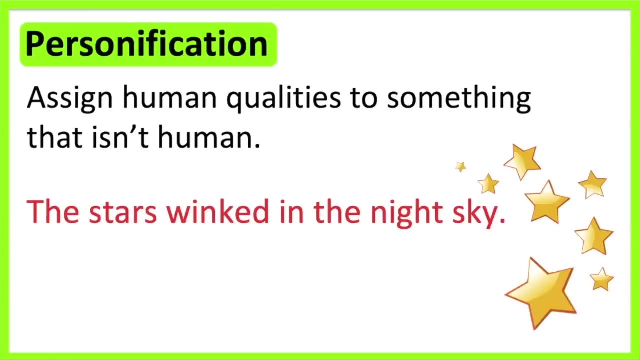 So we know that trees don't have the human quality of dancing. However, this language technique makes the sentence more interesting And creates an image in the reader's mind. It sounds more interesting than just saying the tree is moving in the wind. Another example is the stars winked in the night sky. 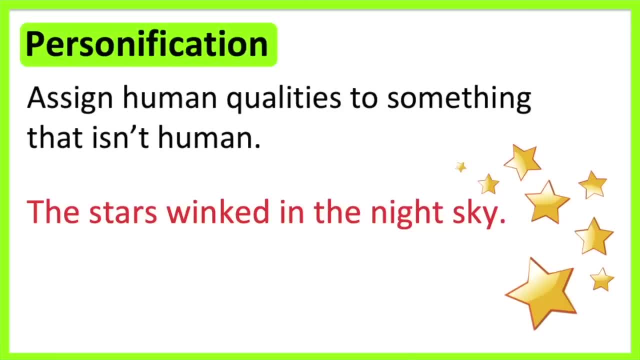 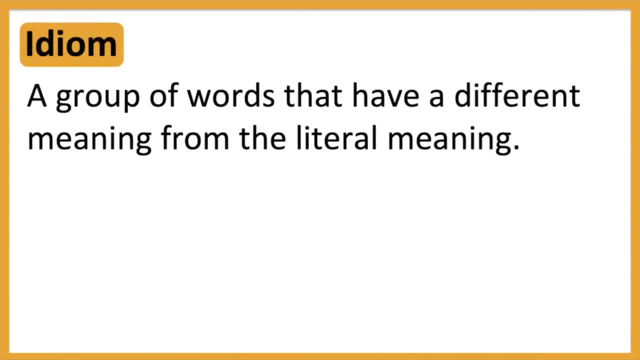 Remember that personification is a figure of speech. Therefore it shouldn't be taken literally, as the words in the sentence convey a different meaning. Idiom- An idiom is a group of words that have a different meaning from the literal meaning. They're interesting ways to get a point across. Idioms are commonly used in 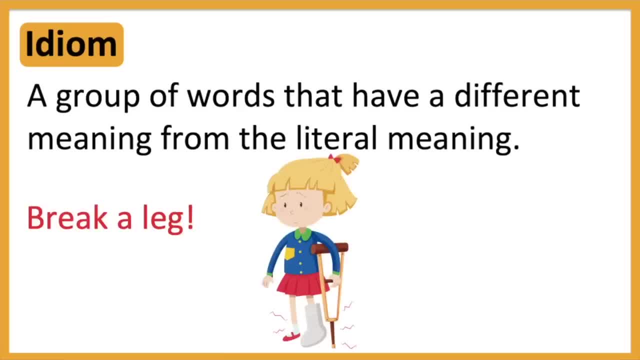 spoken English, For example, break a leg. So this doesn't literally mean break a leg. Rather it means good luck. For example, I could say: I know you can do well on your exam. Break a leg. Another example is the exam was a piece of cake. 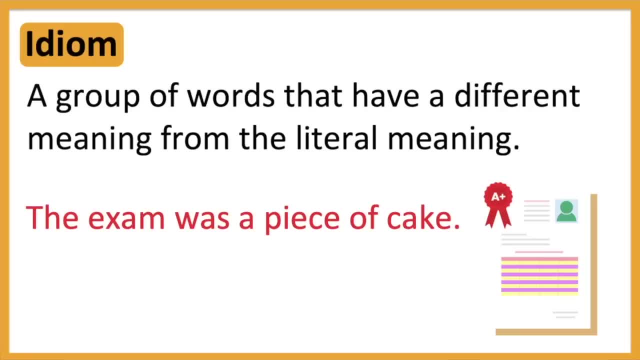 So this means that the exam was very easy. It's important to learn the meanings of different idioms as they're commonly used in everyday spoken English. Remember that an idiom is a figure of speech. This means that it shouldn't be taken literally, as the words in the sentence convey a different meaning. 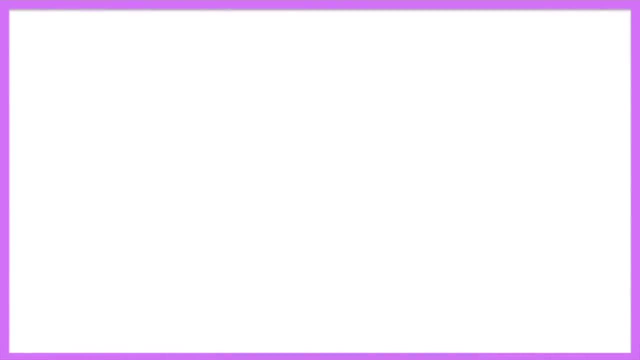 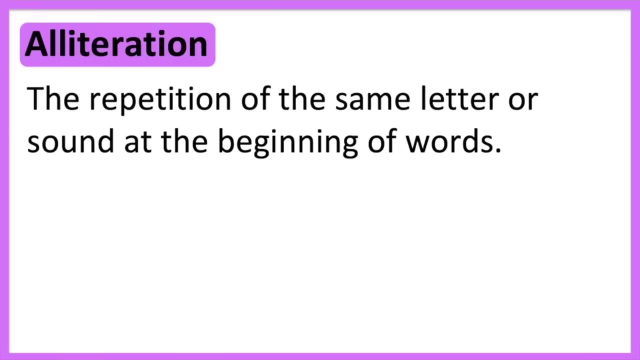 Alliteration. Alliteration is the repetition of the same letter or sound at the beginning of words. Alliteration is used to make writing more interesting for the reader, usually in poems. It also creates a sense of meaning. It's a way of saying: I know you can do well on your exam. 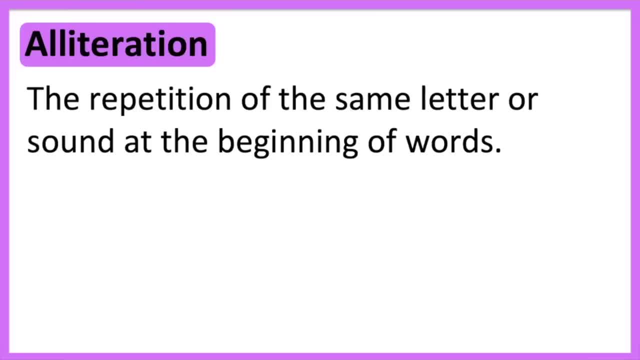 It also creates rhythm and sets the mood. It's important to note that different repeated sounds will have a different effect on the reader. For example, the sly snake slithers slowly in the sand. The repeated S sound in the sentence suggests snake-like qualities, such as the movement of the snake or danger. 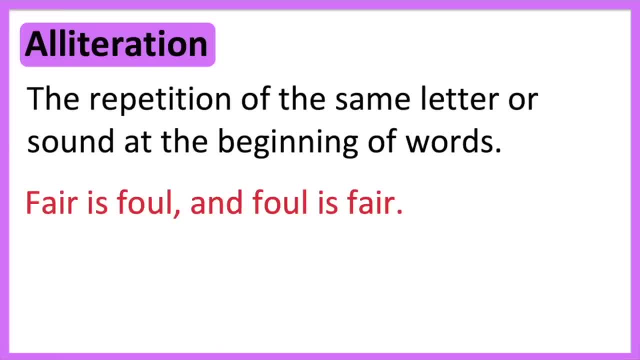 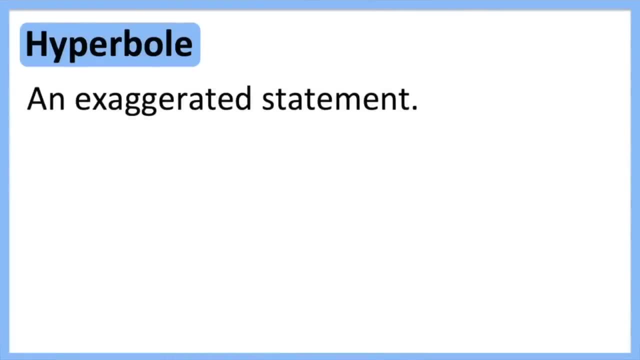 Another example is fair is foul and foul is fair: Hyperbole. Hyperbole is an exaggerated statement. It describes something to be worse or better than it actually is. It's a way to catch the reader's attention and to make writing more interesting. 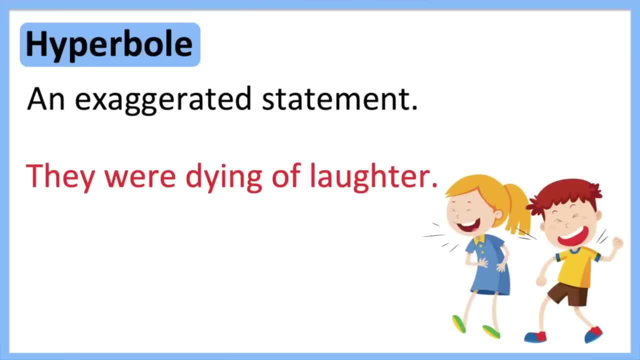 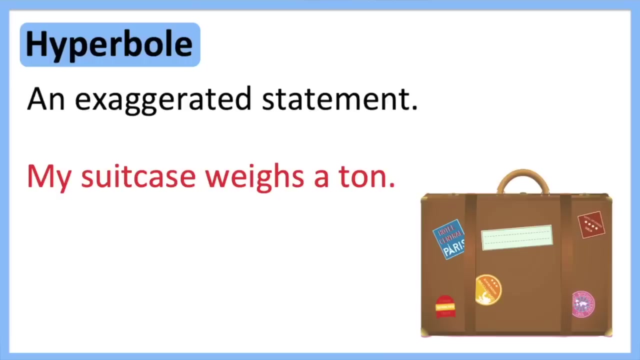 For example, they were dying of laughter. This is an exaggerated statement to emphasize that they were laughing so much. It doesn't literally mean that they were dying. Another example is my suitcase weighs a ton. Again, this is an exaggerated statement to emphasize how heavy my suitcase is. 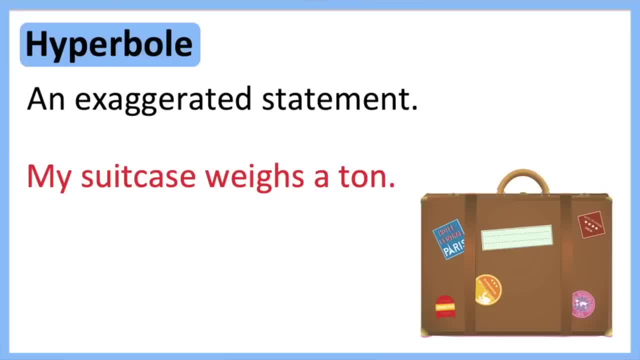 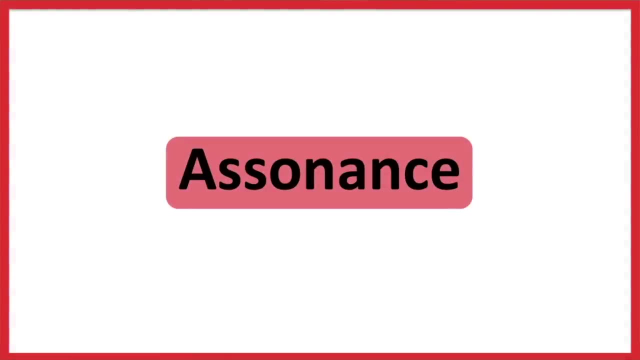 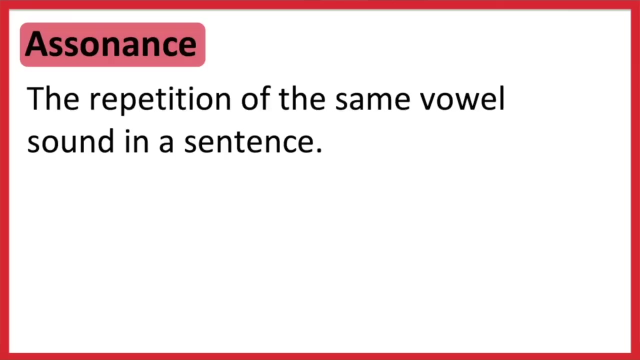 Remember that hyperbole is a figure of speech. This means that it shouldn't be taken literally, as the words in the sentence convey a different meaning. Assonance- Assonance is the repetition of the same vowel sound in a sentence. This language device is used to make writing more interesting and fun for the reader. 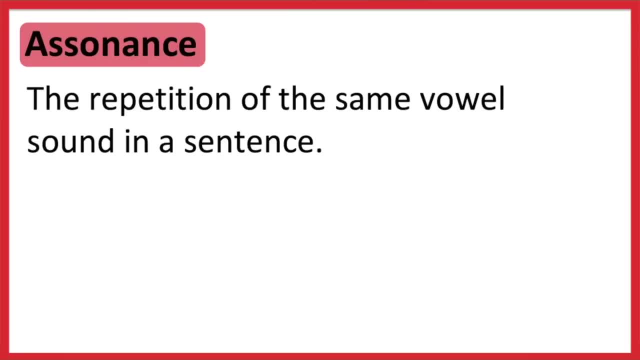 Assonance is usually used in poems. It also creates rhythm, sets the mood and allows the sentences to flow. The vowels are A, E, I, O, U. Each vowel has two sounds: A short vowel sound and a long vowel sound. 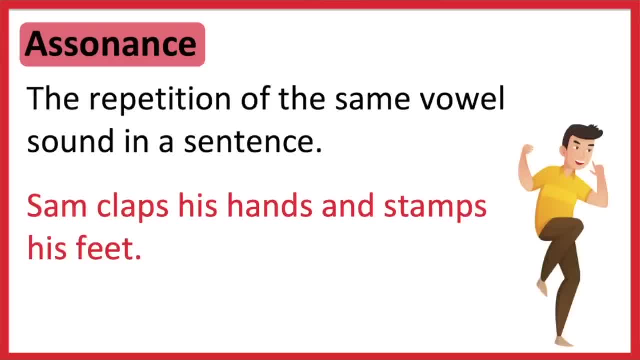 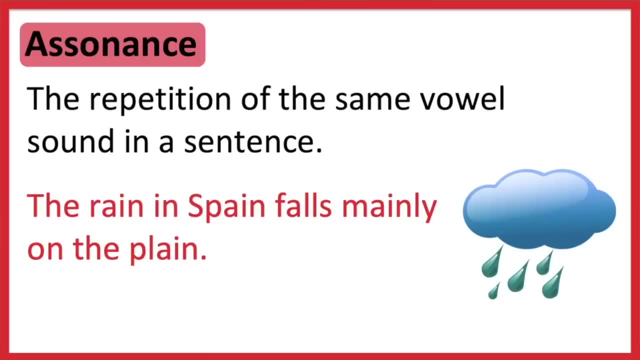 For example, Sam claps his hands and stamps his feet. In this example, the short vowel A is repeated. Another example is The rain in Spain falls mainly on the plane. In this example, the long vowel, sound A, is repeated. Oxymoron. 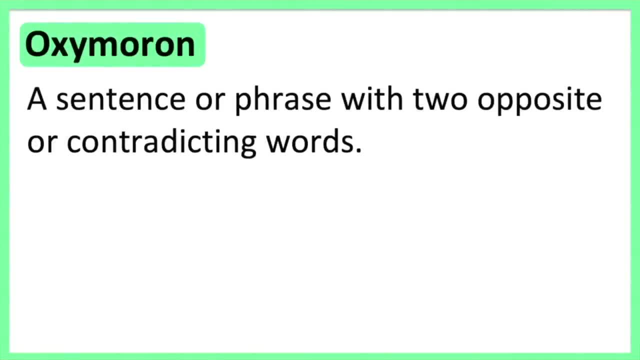 An oxymoron is a sentence or phrase with two opposite or contradicting words. Oxymorons are used to interest the reader and causes the reader to pay attention to what they're reading. It also adds some playfulness in the sentence. 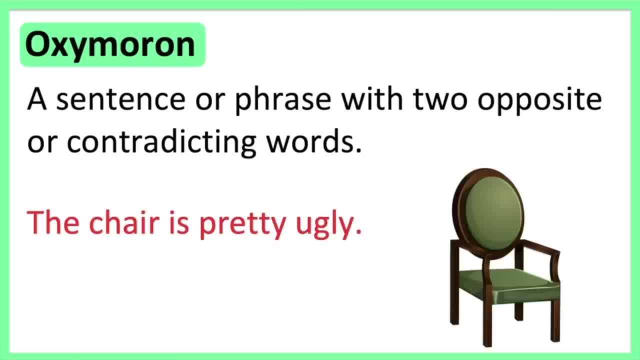 For example, The chair is pretty ugly. Pretty and ugly are opposites. Another example is Assonance: Alex is seriously funny. Serious and funny are opposites. Remember that an oxymoron is a figure of speech. This means that it shouldn't be taken literally. 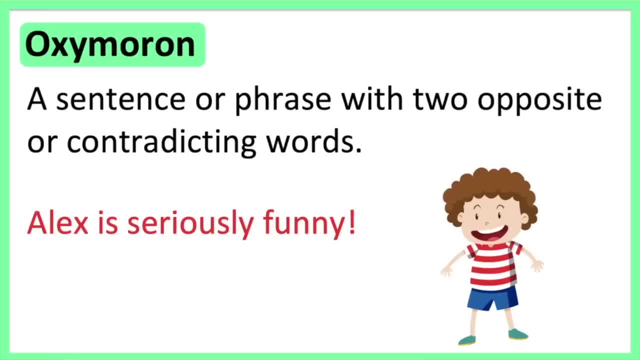 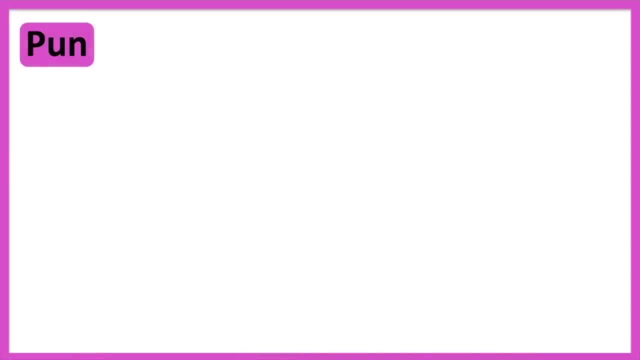 as the words in the sentence convey a different meaning. Pun A pun is a humorous use of words that convey a natural, natural meaning. Puns are commonly used in everyday spoken English. We can also use puns in writing to make our writing more interesting to the reader. 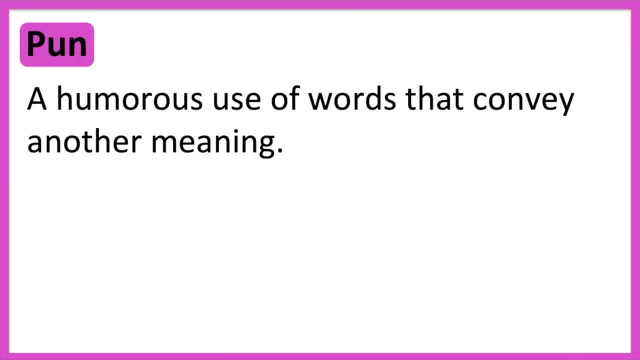 and to create a humorous effect. For example, I like kids, but I don't think I could eat a whole one. In this example, the word kid has two meanings. It can refer to a child or a young goat, So this pun adds a humorous effect to the sentence. 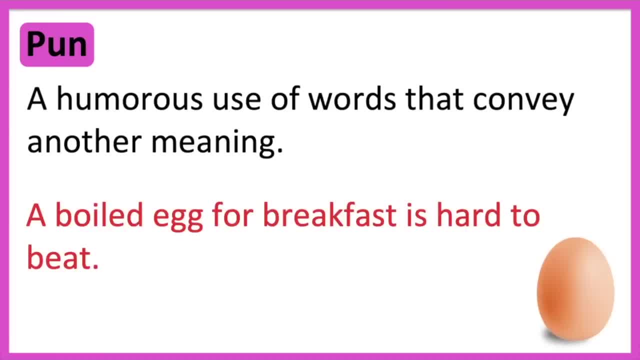 Another example is A boiled egg for breakfast is hard to beat. In this example, the word beat has two meanings. Remember that a pun is a figure of speech. This means that it shouldn't be taken literally, as the words in the sentence convey a different meaning.